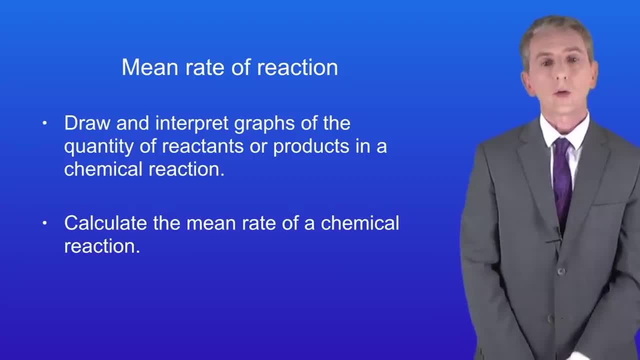 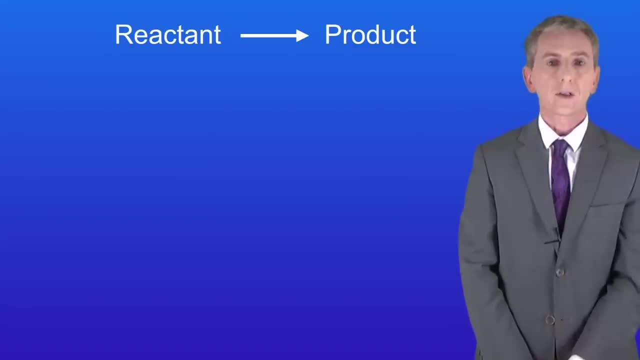 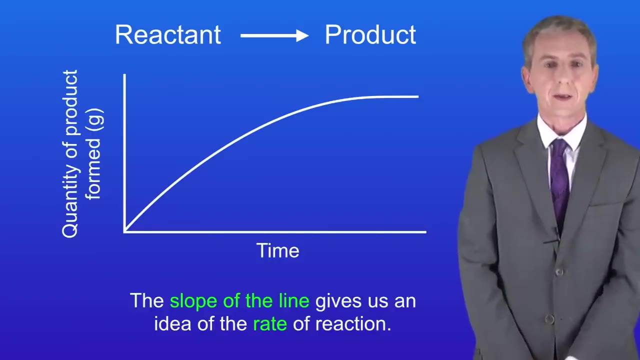 a bit tricky, but the actual ideas are relatively straightforward. I'm showing you a chemical reaction here. As you can see, the reactant is turning into the product. If we plot the quantity of product formed against time, then we get this graph. Now the slope of the line. 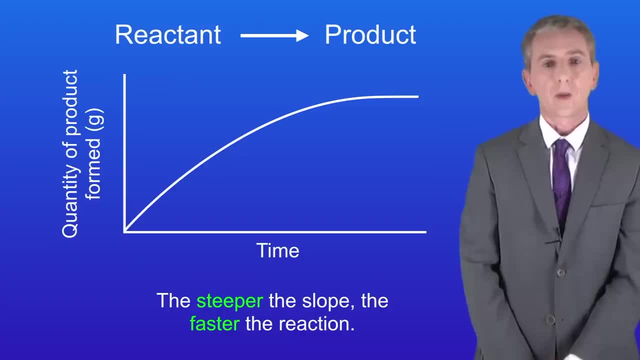 gives us an idea of the rate of reaction. The steeper the slope, the faster the reaction. So, as you can see, initially the reaction is very fast. We can tell that as we're making a lot of product in a short amount of time. That's because we've got a large number of 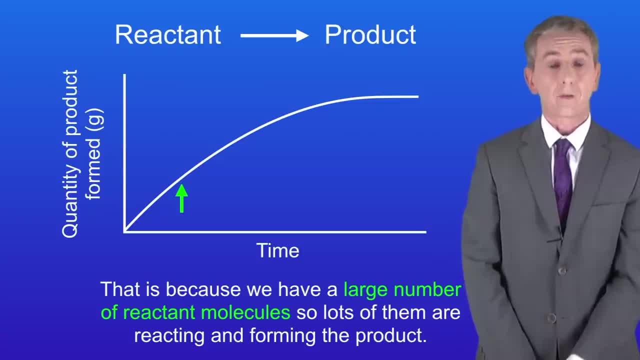 reactant molecules, So lots of them are reacting and forming the product. Gradually the slope of the line becomes less steep. This tells us that the reaction is slowing down. In other words, the rate of the reaction is decreasing. Now that's because a lot of the reactant molecules have already 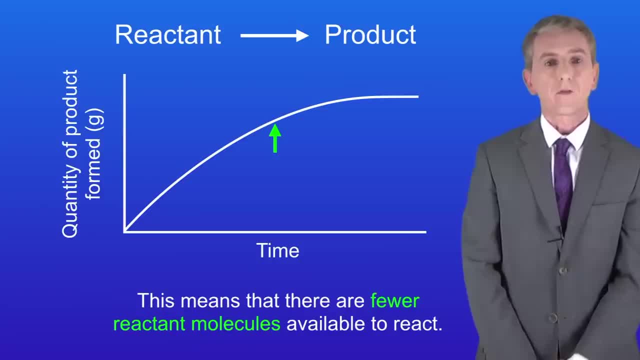 reacted and turned into product. This means there are fewer reactant molecules available to react. At the end we can see that the slope of the line is now zero. In other words, the line is flat. This means that at this point the reaction has stopped, And that's because all of the 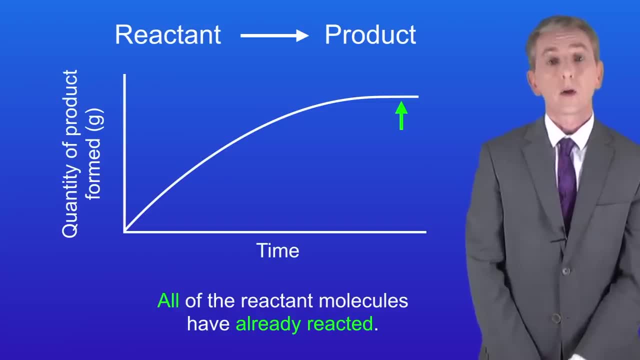 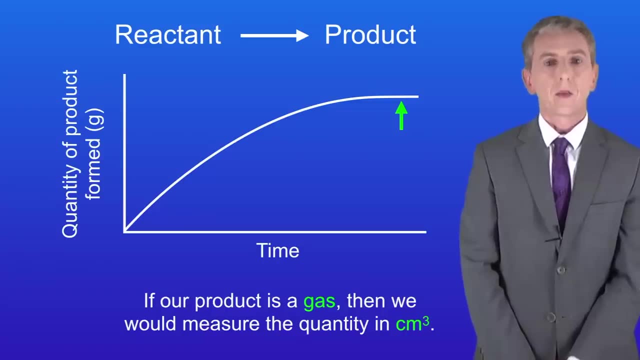 reactant molecules have already reacted. Now you'll notice that in this reaction we're measuring the quantity of product formed in grams. But if our product's a gas, then we'd measure the quantity in centimetres cubed. So, as we've seen, we can measure the quantity of product formed in a chemical reaction. 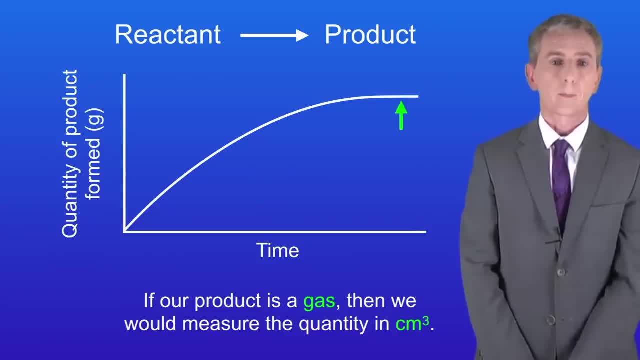 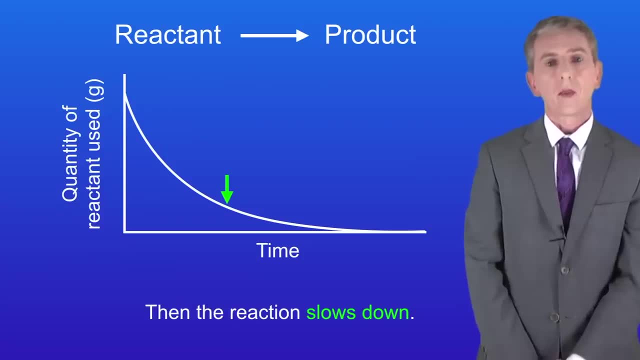 Another way of looking at the rate is to measure the quantity of reactant used. In this case, the graph looks like this. Again, we can see that initially the rate is fast, Then the reaction slows down and finally the reaction stops. Now in the exam you could be asked to calculate the mean rate of a reaction. So we're going. 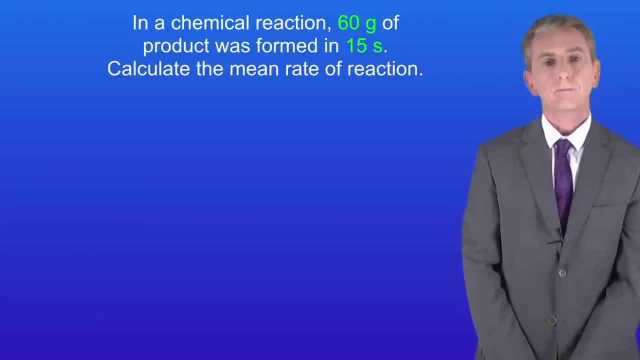 to look at that now. Here's a sample question. In a chemical reaction, 60 grams of product was formed in 15 seconds. Calculate the mean rate of reaction Now. to do this we use this calculation. The mean rate of reaction equals the quantity. 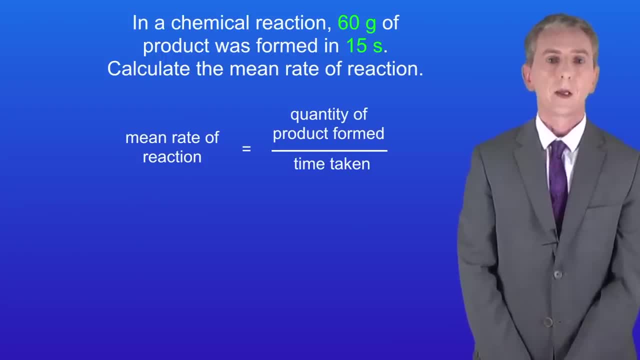 of product formed divided by the time taken. The quantity of product formed is 60 grams and the time taken is 15 seconds. 60 divided by 15 gives us a mean rate of reaction of 4 grams per second. Here's a question for you to try.